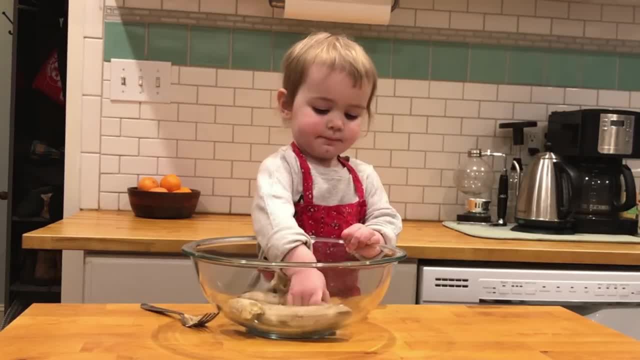 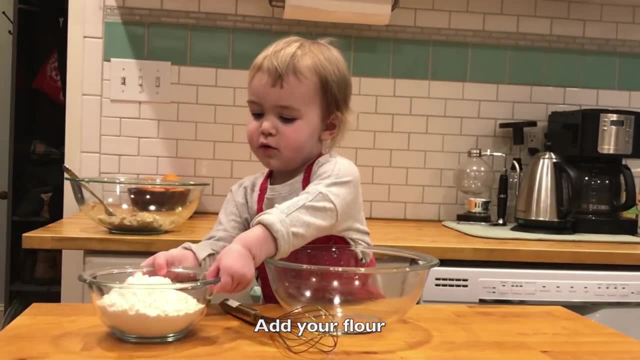 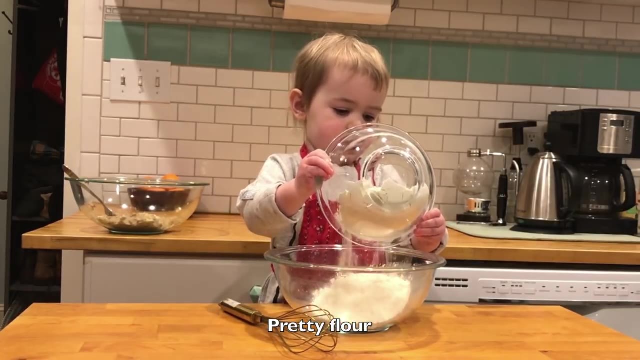 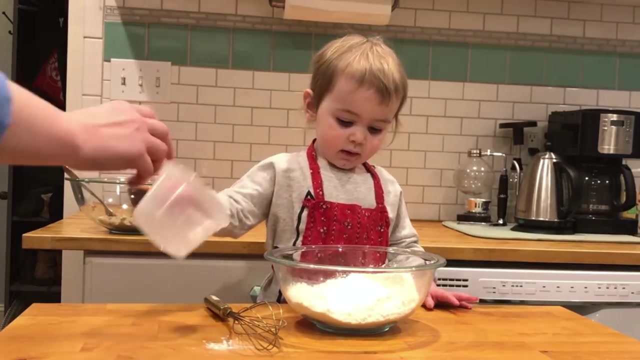 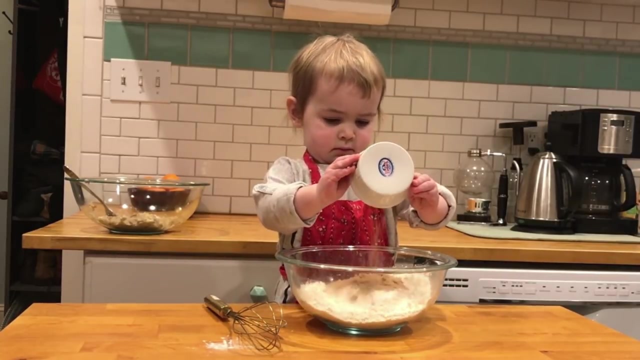 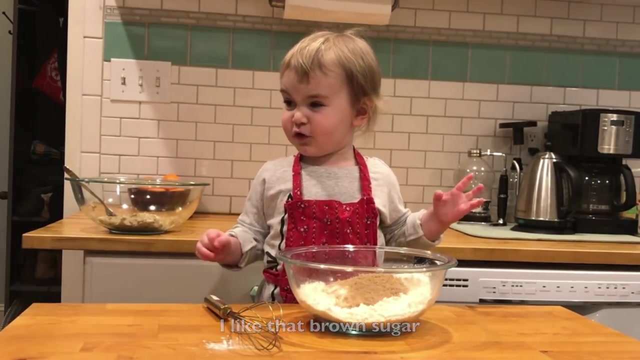 Now I'm going to eat them. Set that aside. Add flour, Pudding flour And white sugar. It's so sparkly, So sparkly. I like that brown sugar. I like that brown sugar. I like that brown sugar. 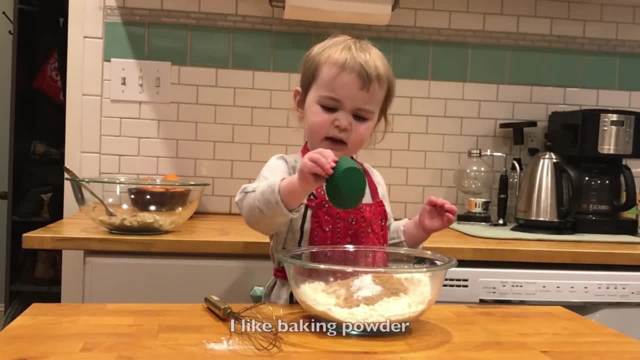 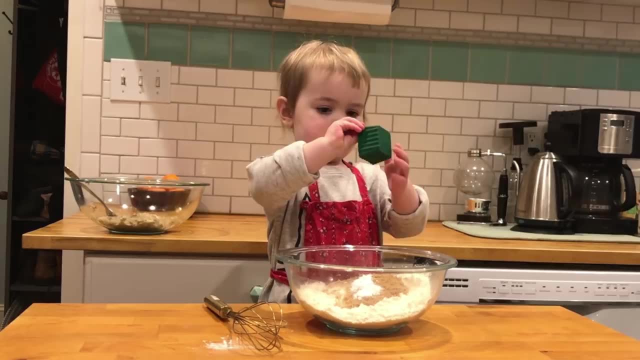 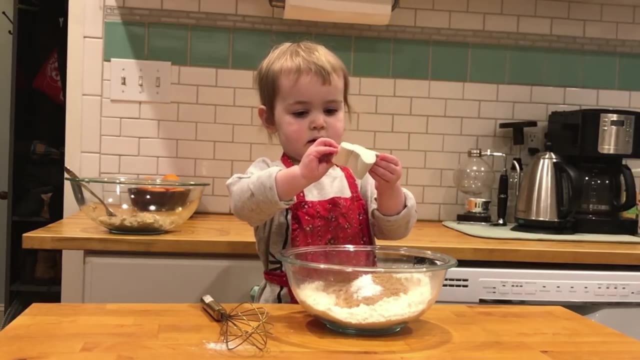 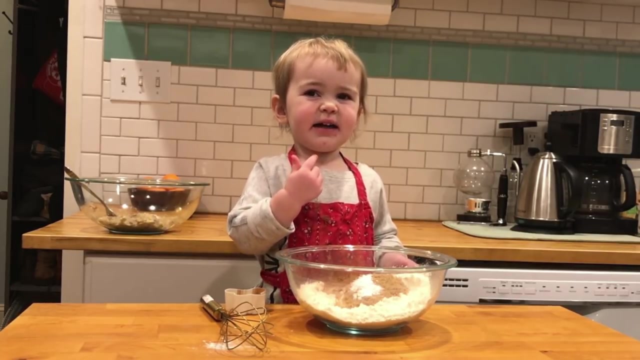 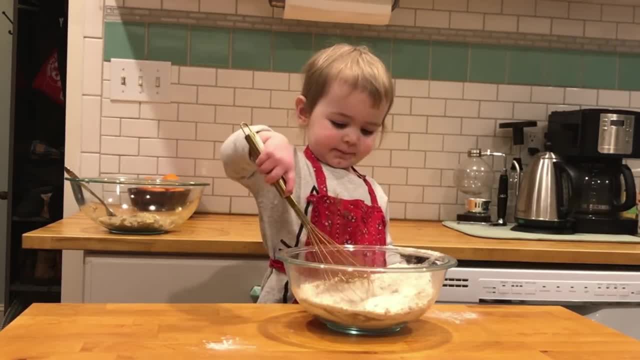 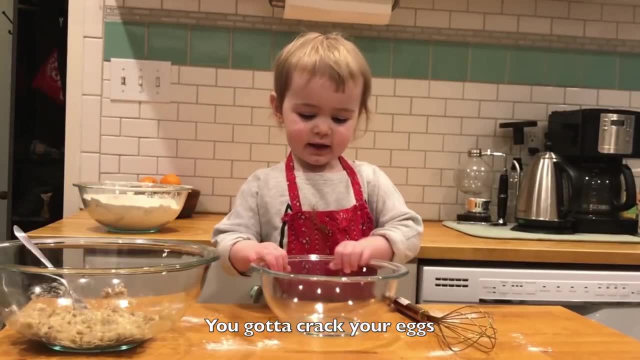 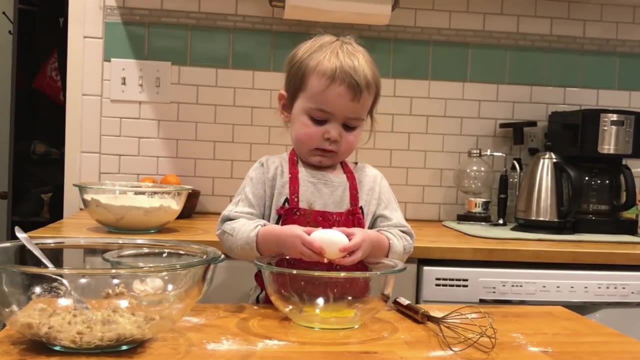 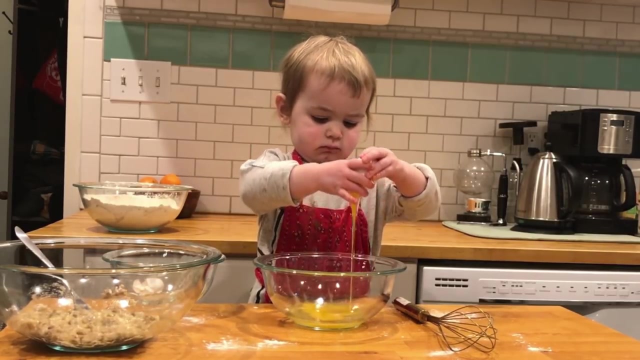 Add baking powder Mix, adhesive Mix, Mix, Mix, Mix, Stir, Stir, Stir. I usually know what's protestant. Place it to the side. You've got to pop your eggs, voi тво. Add oil. 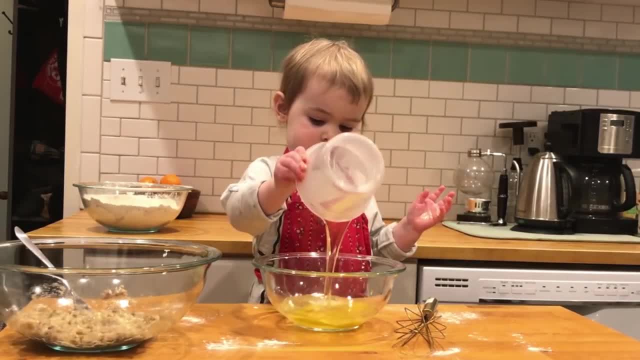 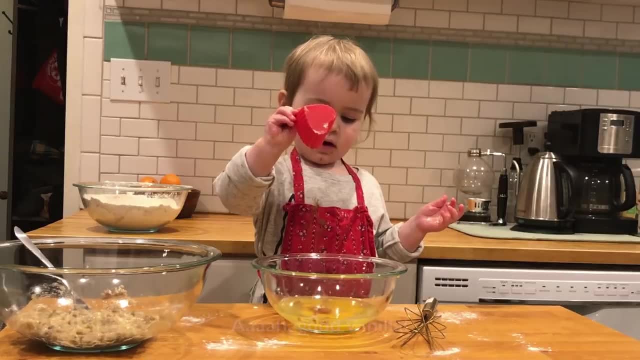 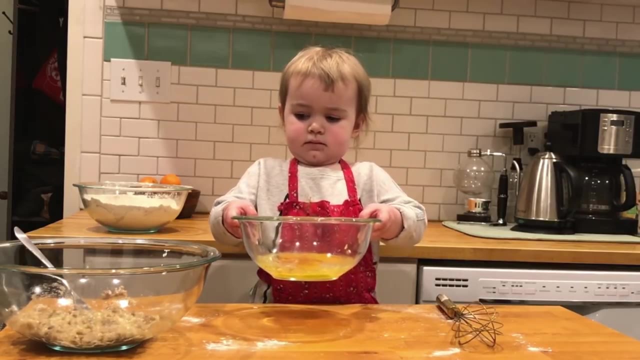 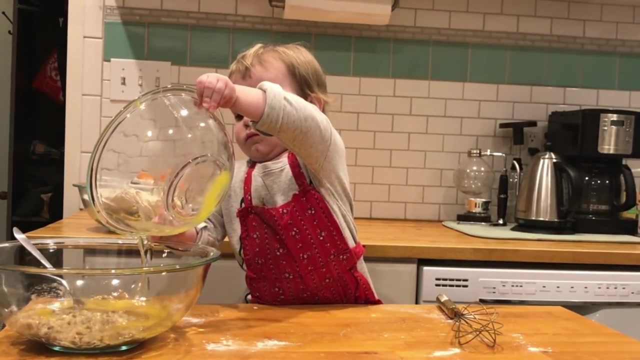 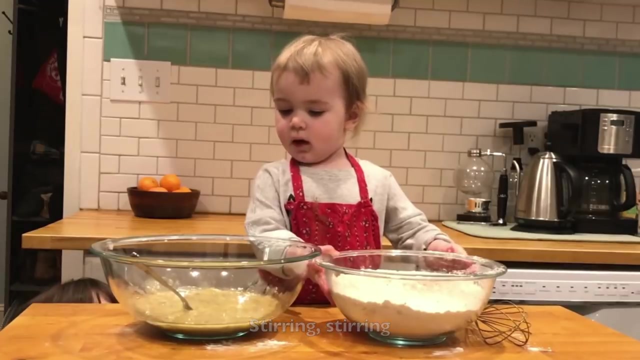 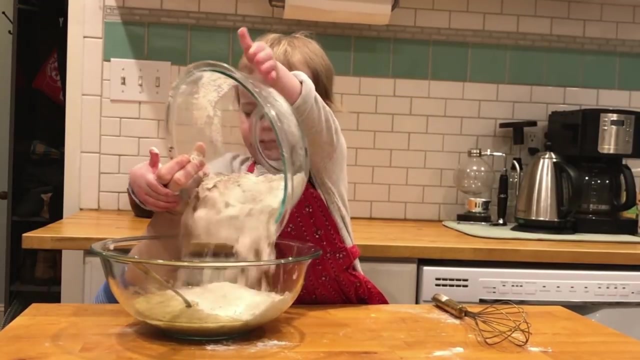 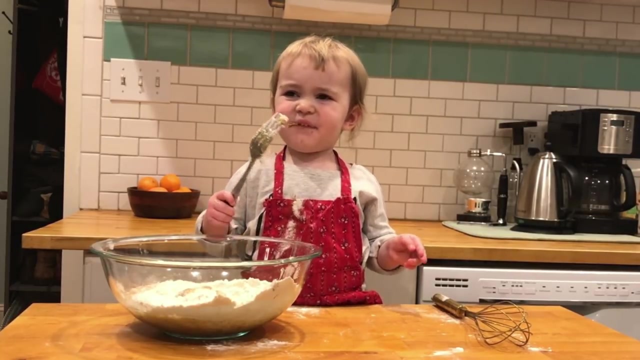 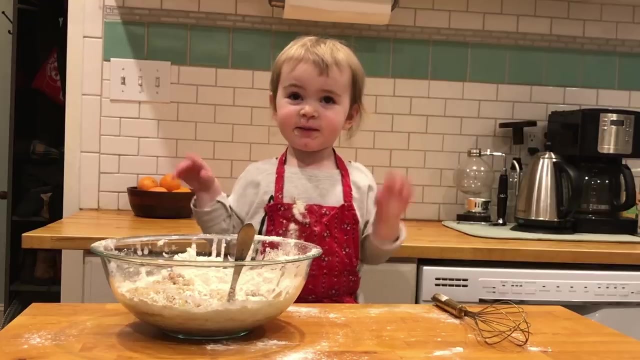 Add oil. Good for nimmer. Good for nimmer. Good job, What's missing? Soon soon, I'm going to do this myself. Good job, self. Don't eat the batter. Oops, It's time for my favorite, favorite part.